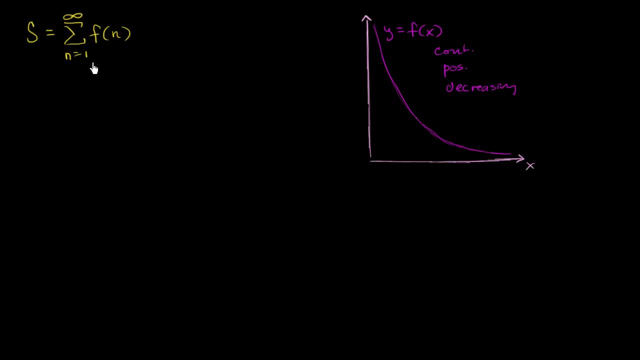 exactly what it converges to, and instead we're going to have to do it using a computer or by hand, And in those cases it's good to know how good our estimate is, And we also want as good of an estimate as possible. 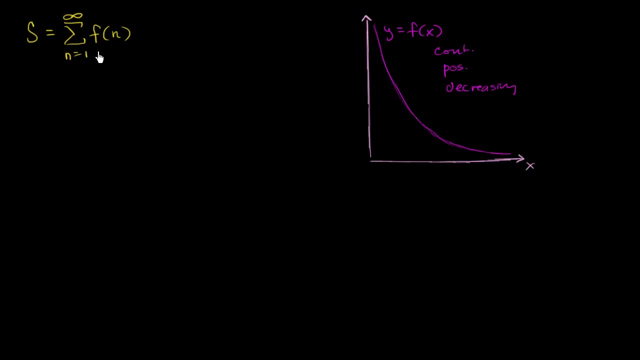 with as little computation as possible. So let's think about how we can do that. Well, the way to tackle it, you could imagine, is: let's split this up, this infinite sum. let's split it up into the sum of a finite sum. 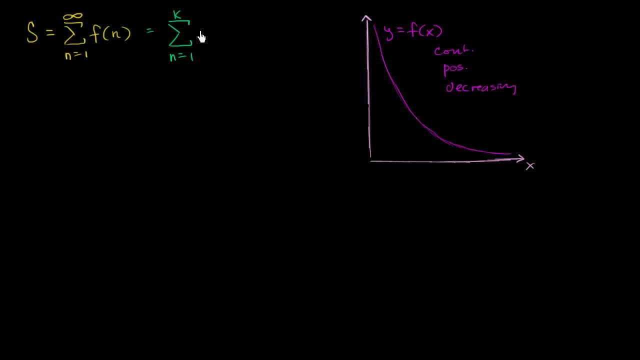 So let's say the first k terms. So n equals one to k of f of n. So this is very, this is very computable. If k is low enough, you could probably even, and if f is a simple enough function. 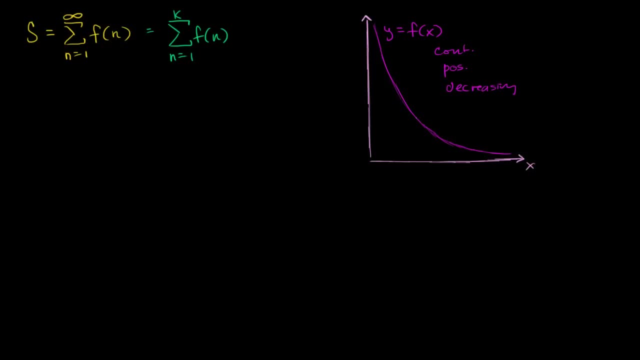 you could probably do this by hand, but you could definitely do this with a computer, And then it's going to be that plus an infinite, plus another infinite series. But now you're going to pick up at k plus one, the k plus one-th term. 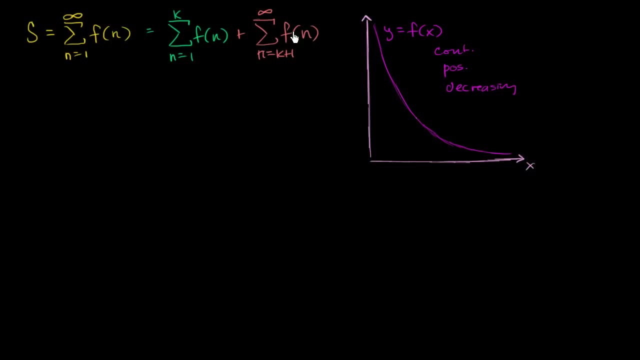 and you're going to go to infinity of f, of n. So if we could put some bounds on this, then that'll allow us to put some bounds. it'll allow us to put some bounds on this right over here, which is the sum of the partial sum. 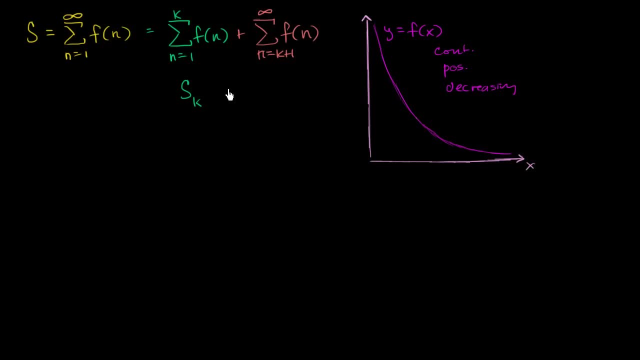 of the partial sum of the first k terms and the remainder that we get after to get us to the actual value. So you could see what kind of what's left over after we take that partial sum. And this will be. this is easier to write for me than this right over here. 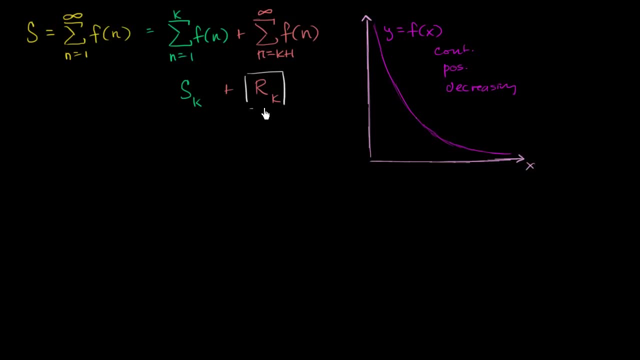 So the key is: can we come? can we come up with some bounds for this? And to do that, I'm going to go to this graph and use some of the same arguments that we used, or the same conceptual ideas we used, for the integration test. 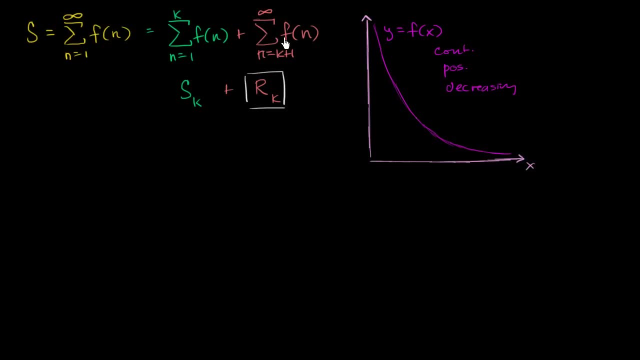 If we there's two ways to conceptual. there's two ways to conceptualize what the sum represents relative to this graph. As we'll see, it can represent an overestimate of the area between some x value and infinity, and it could represent the underestimate. 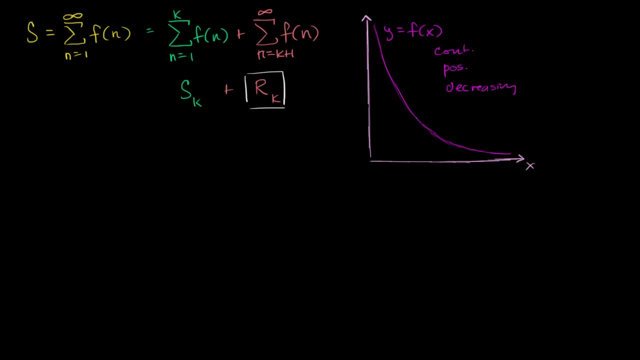 of a different region. So let's look at that. So let's first think about, let's first think about the underestimate. Let's think about the underestimate. So if this right over here, let's say that this right over here is k. 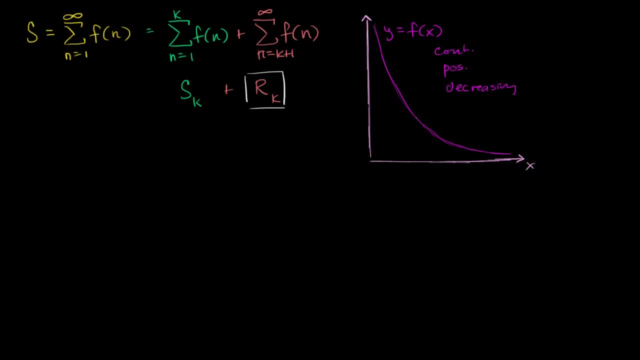 actually let me do it in a color that you let's. let me do it in that. let me do it in a yellow color. So let's say that this right over here is k. this is k plus one. this is k plus. 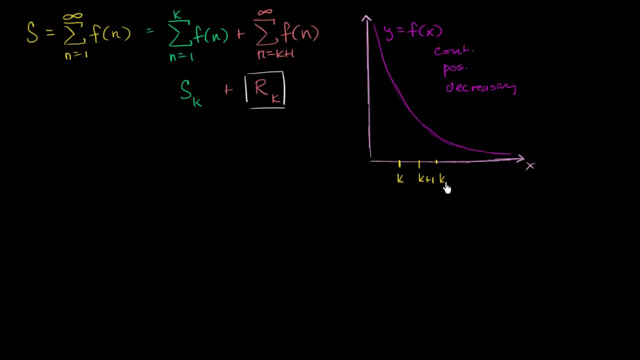 that's let's do. this is k plus two, k plus two, k plus three, on and on and on. So one way to conceptualize this sum right over here is it could be the sum of the following rectangle. So the first term is this area. 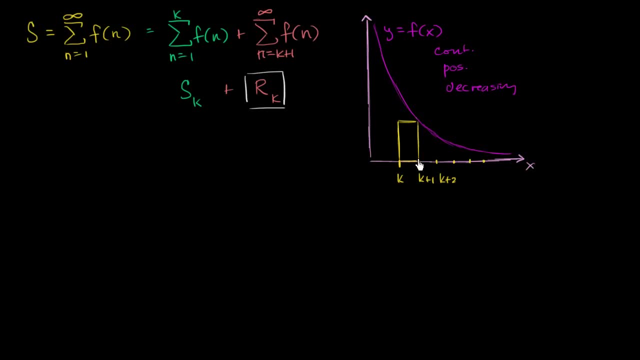 the area of this first rectangle, because this area's height, or this rectangle's height, is f of k plus one, is f of k plus one, and its width is one. so f of k plus one times one, its area is just going to be f of k plus one. 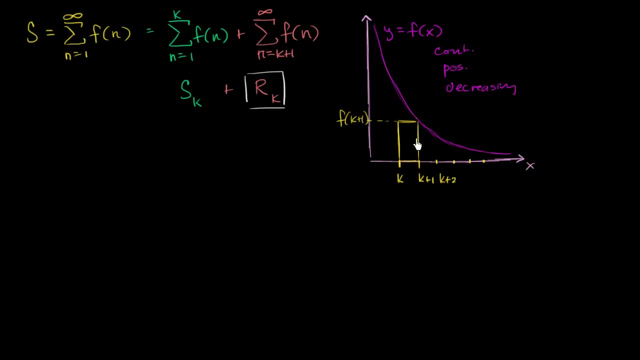 which is exactly this first term right over here, when n is k plus one. And then the second term by the same argument could represent the area of this rectangle. The third term could represent the area of this rectangle. The fourth term could represent the area of that rectangle. 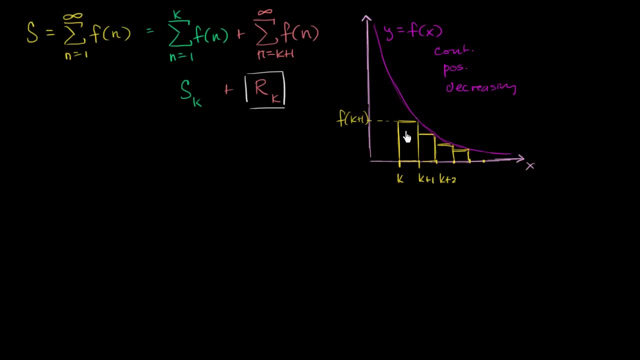 And we could just keep going on and on and on. And so, what are the? what is the sums of these areas, of these rectangles, What are the sum of these terms representing? Well, you could view it as an estimate. you could view it as an estimate. 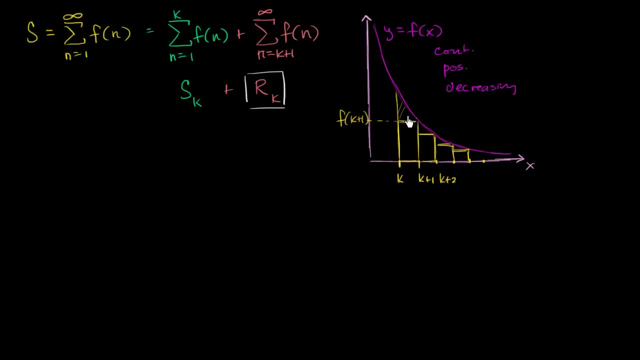 of the area under the curve between x equals k and x equals infinity, but it's going to be an underestimate. Notice, these are all completely contained in that area. So one way to think about it is that our r sub k is less than or equal to its underestimate. 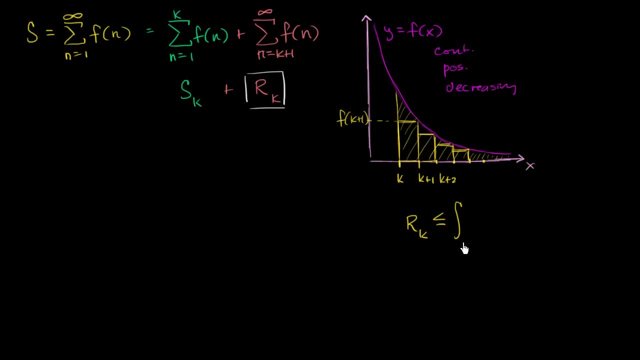 for the area between x equals k and infinity of f, of x, dx, So that essentially puts an upper bound. That puts an upper bound on us, And this is already interesting, because now we can already say: if s, so we know that s is equal to this. 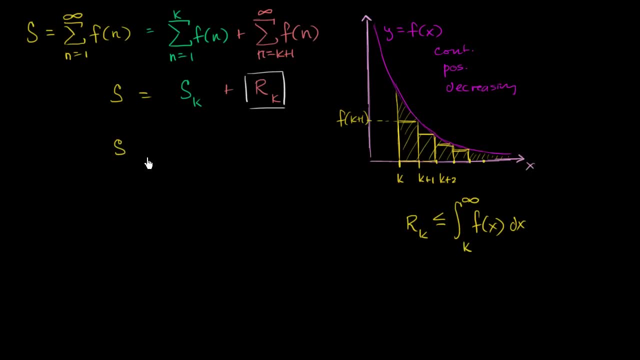 Now, if this is less than this thing, right over here we can say that s is equal to this. So s is going to be less than or equal to our partial sum plus this thing, plus the improper integral from k to infinity, of f, of x, dx. 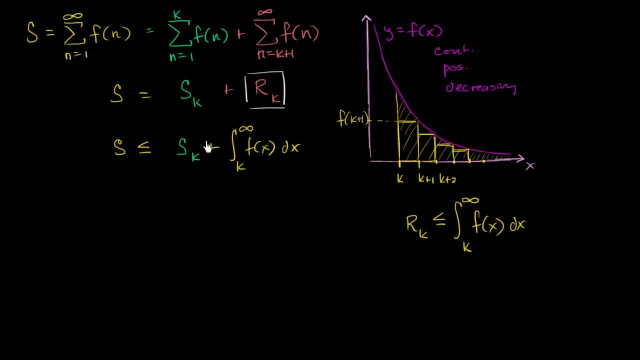 Notice if this is equal to this. and now, since this is less than this, this must be less than what we have on the right-hand side. So, just like that, if we're able to compute these two things- and we are often able to compute these two things- 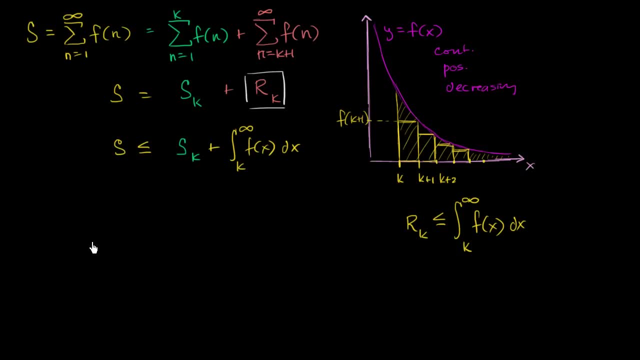 we're able to put an upper bound on our actual sum. Now what about placing a lower bound on it? Well, we could conceptualize the same sum, the same r sub k. Instead, we can conceptualize it this way, where the first term here represents not this rectangle: 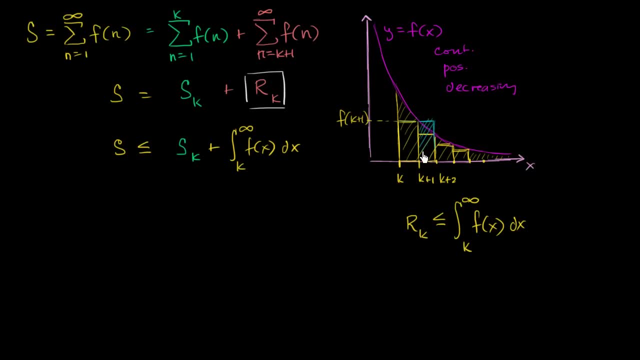 but it represents this rectangle. Notice it has the same height, but it's just shifted over one to the right. The second term represents this rectangle. The third term represents this rectangle. Why does that make sense? Well, the area of this first rectangle. 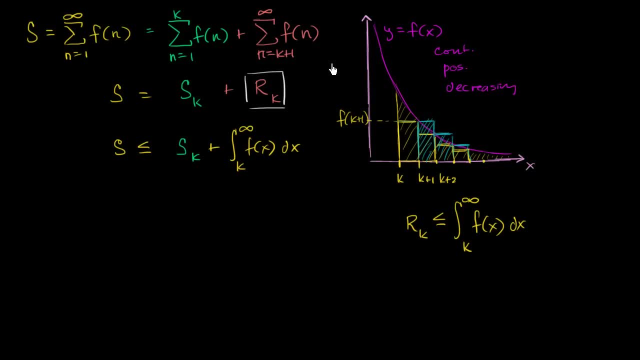 this is going to be it's height, which is f of k plus one. f of k plus one times its width, which is this one. so it's just going to be f of k plus one. So this is the area. here is the first term. 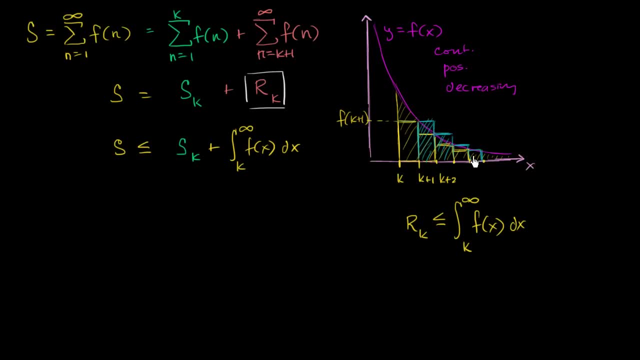 the area here is the second term. area here is the third term. the area here is the fourth term. One way to think about it: we just shifted all of those yellow rectangles- one to the right, But now this is approximating a different region. 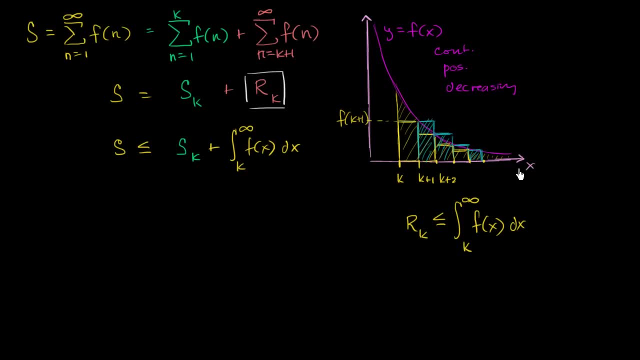 This is approximating the area under the curve, not from k to infinity, but from k plus one to infinity, and instead of being an underestimate, it's an overestimate. Now the curve is contained within the rectangles, So we could say that r sub k. 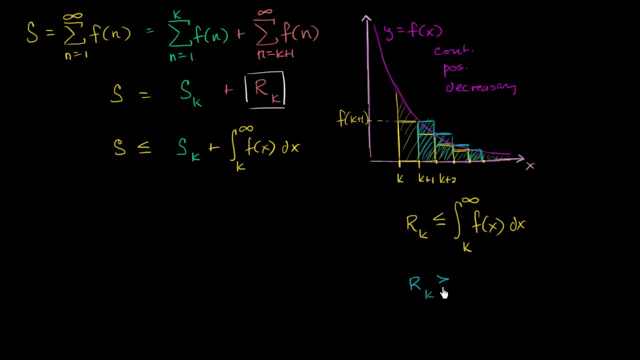 in this context, when we conceptualize it this way, is going to be greater than or equal to the improper integral, not from k, but from k plus one, from k plus one to infinity, f of x, dx. And what does that allow us to do? 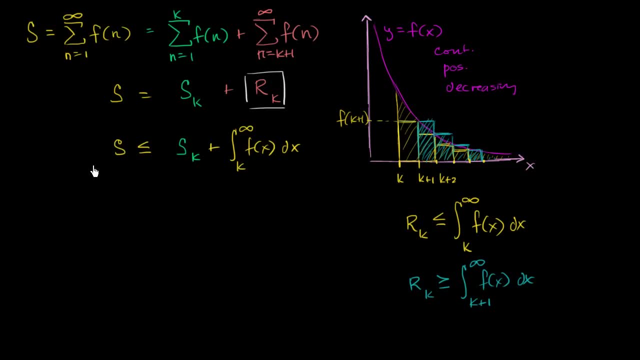 Well, this places a lower bound on this, which will also place a lower bound on this. If this is greater than that, then this is going to be greater than this. replaced with the improper integral, So we can write that So s is going to be greater than or equal to. 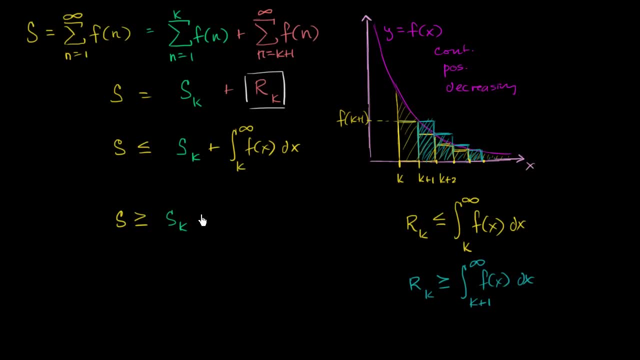 s sub k plus plus the improper integral from k plus one to infinity f of x, f of x, dx. Now you might be saying, hey, Sal, this looks all crazy. you have all this abstract notation here. you've got to introduce an integral sign. 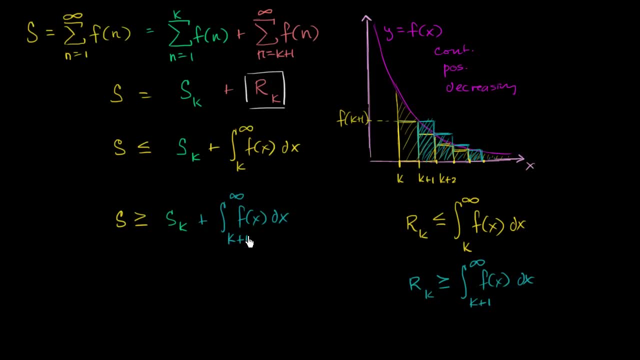 this seems really daunting, but, as we'll see in the next few videos, these are actually sometimes fairly straightforward to compute. This can be very straightforward to compute if our k is not too large. if it's even large, a computer can do it.